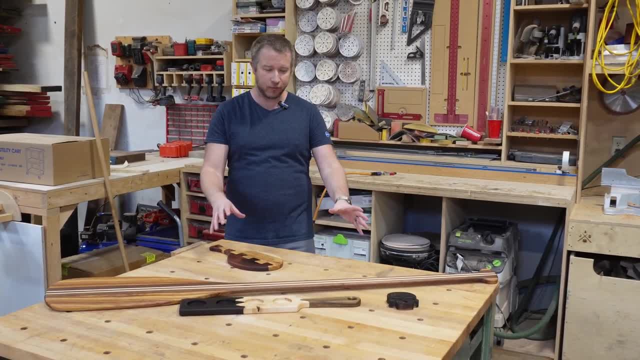 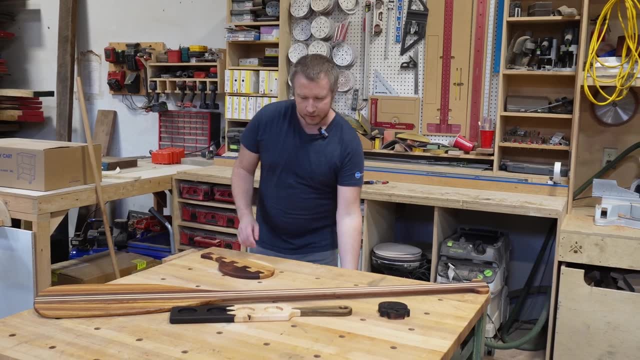 Hey guys, today we've got five projects in five minutes. We've got these four plus this one, which is pretty sweet and pretty easy to do, And you're going to want to stick around for this one. This one's my favorite. It uses our 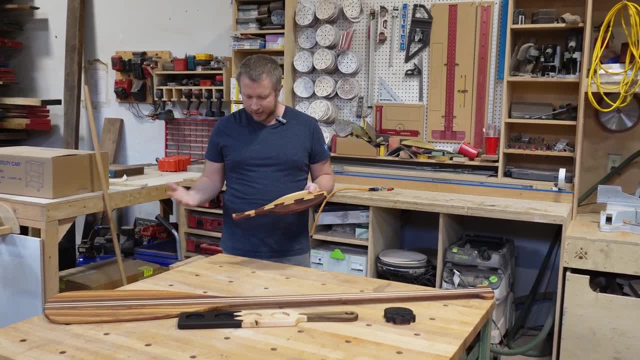 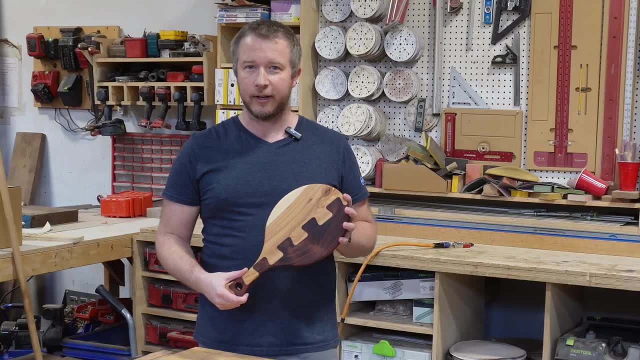 new dovetail template, which is kind of a one-of-a-kind template that you can't really get anywhere else, and it creates some really unique looks. So stick around: Lots of value here, crammed into five minutes. Let us know what your favorite project is. 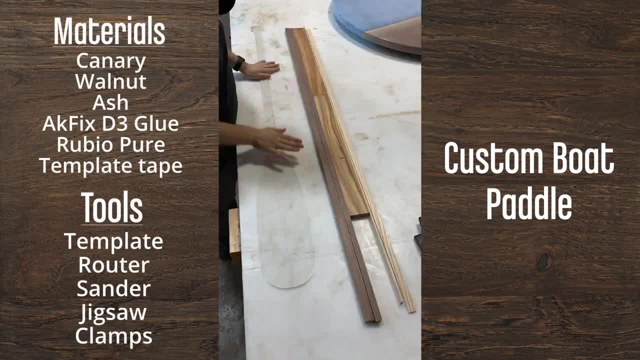 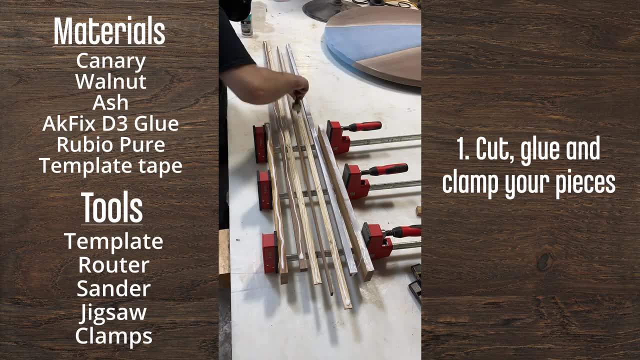 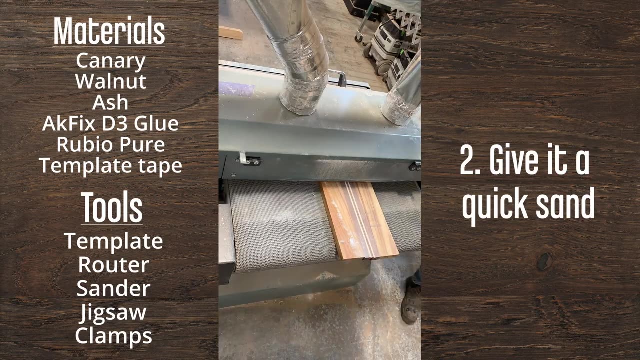 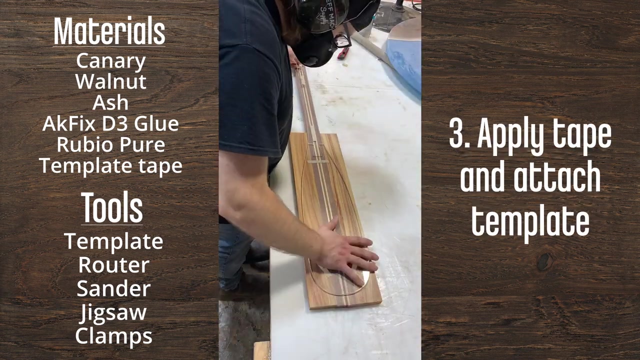 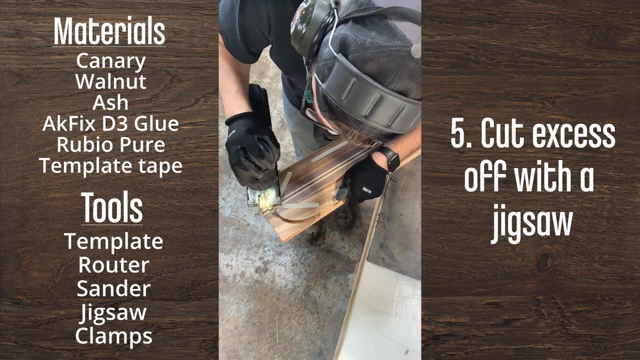 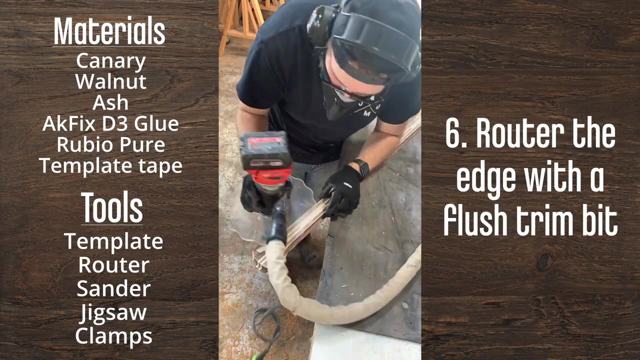 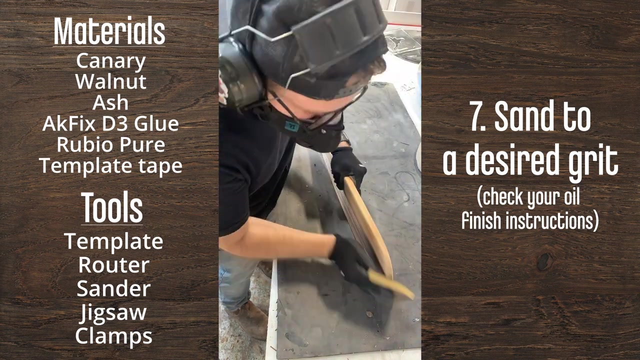 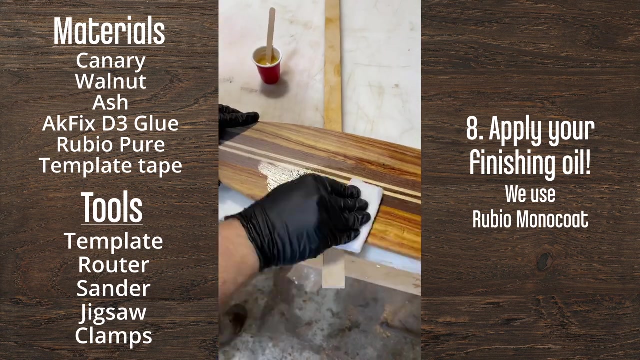 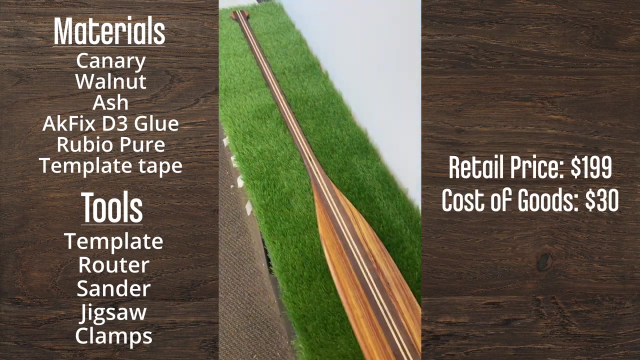 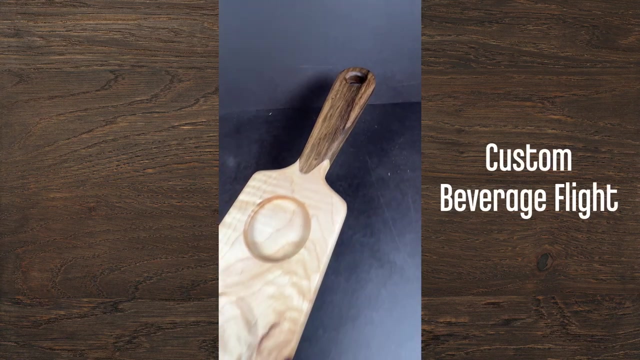 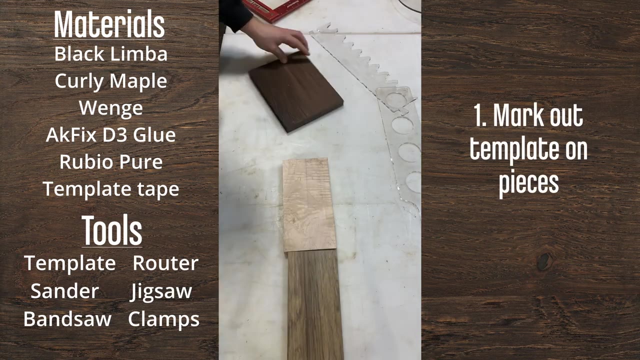 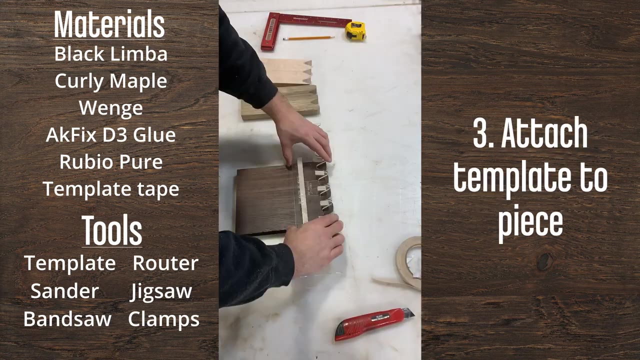 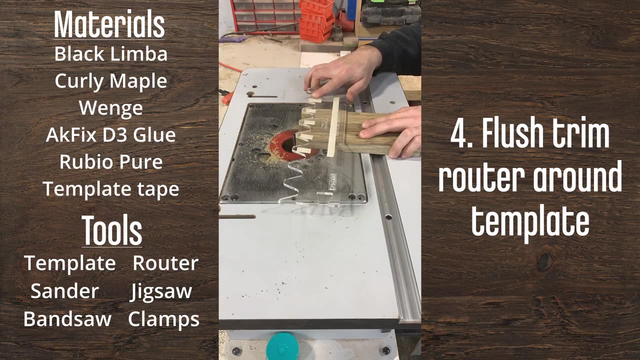 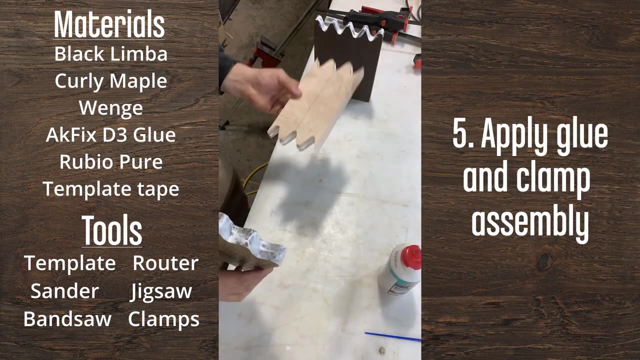 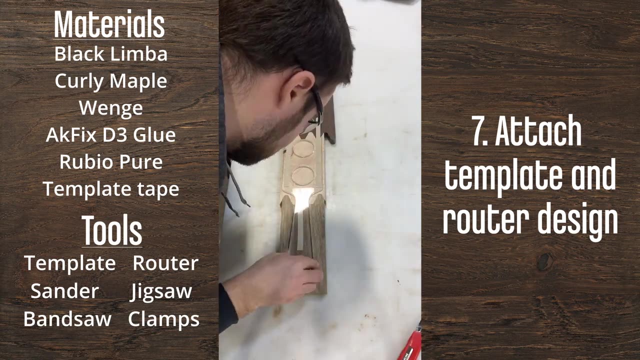 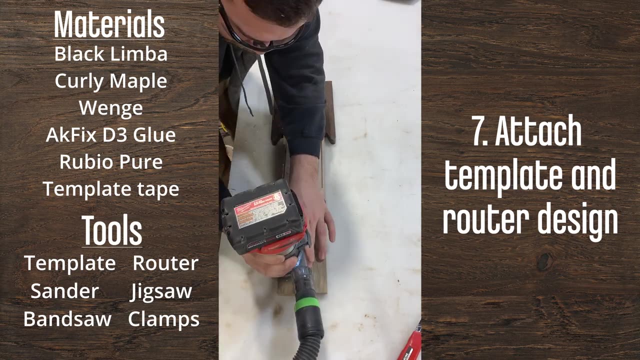 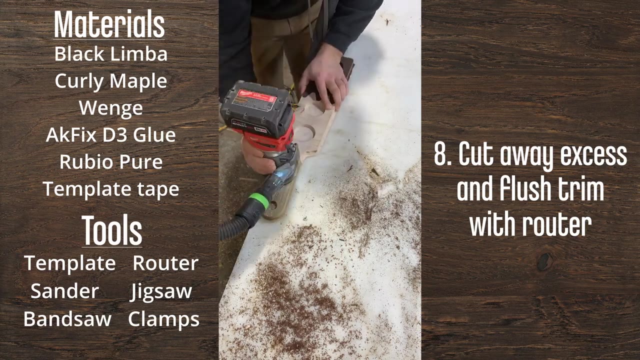 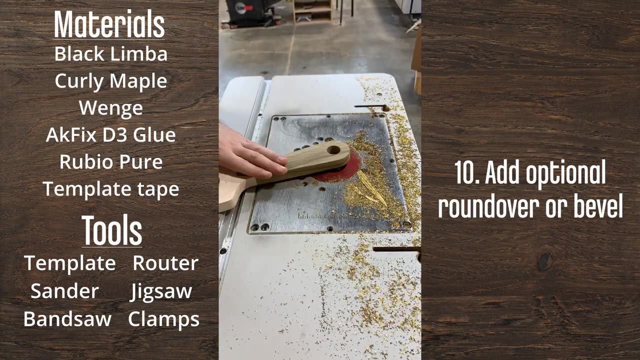 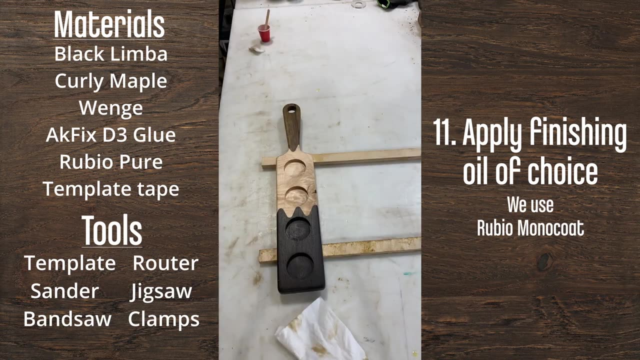 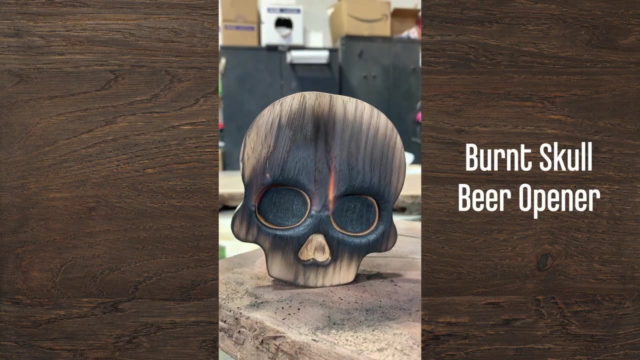 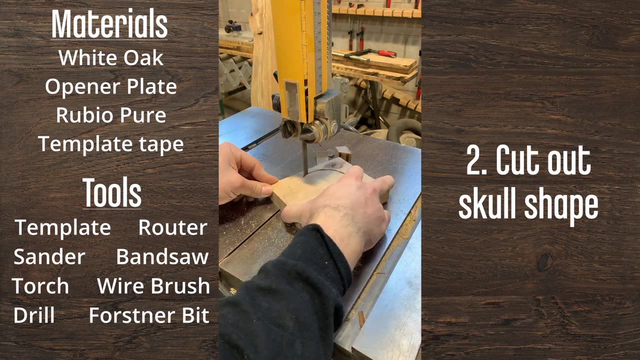 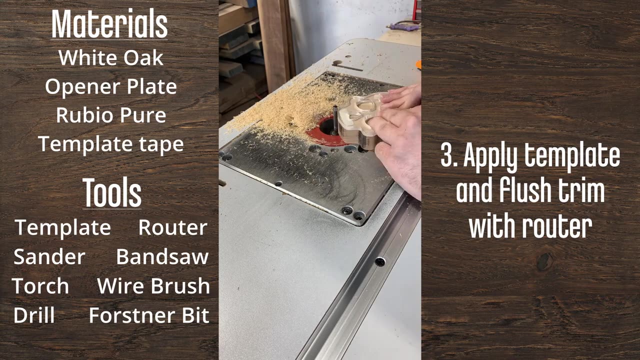 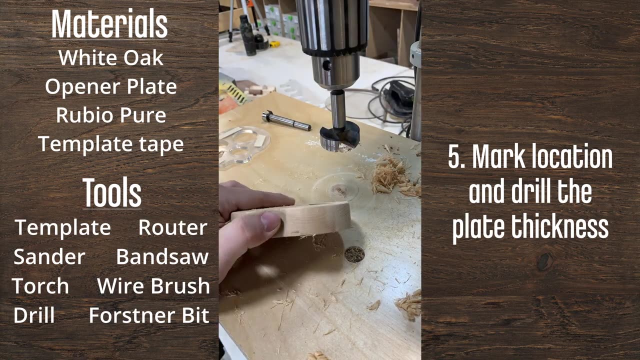 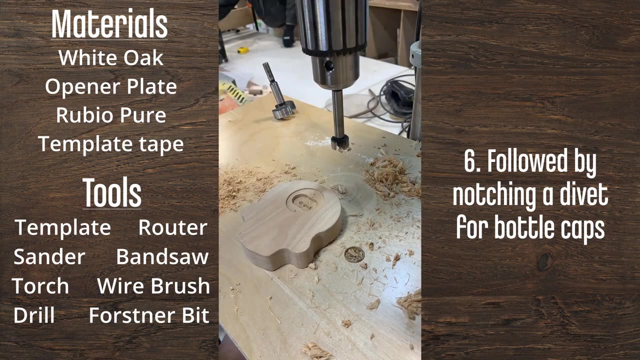 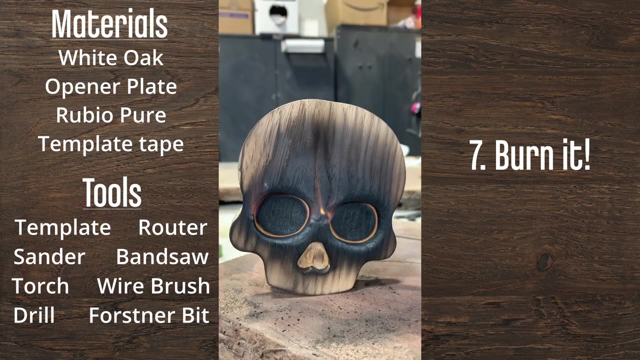 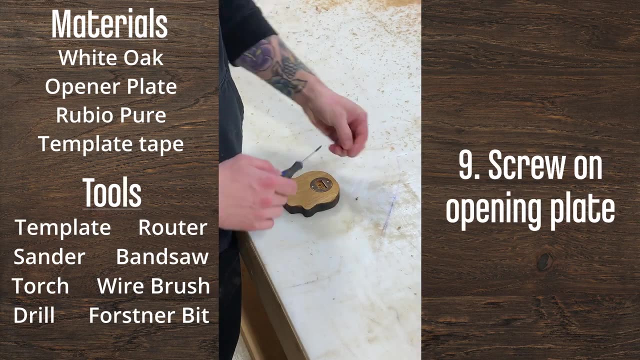